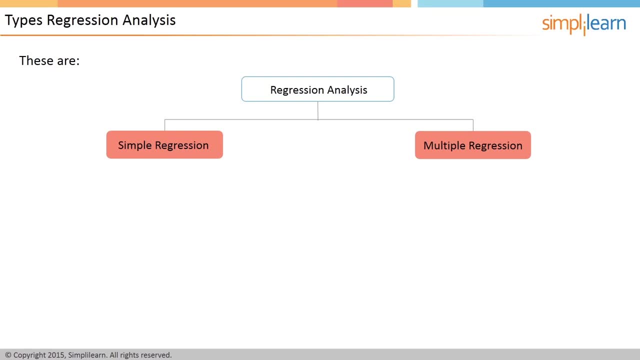 regression to model the relationship between two or more variables. Simple linear regression considers one quantitative and independent variable, x, to predict the other quantitative but dependent variable y. Multiple linear regression considers more than one quantitative and qualitative variable to predict a quantitative and dependent variable y. 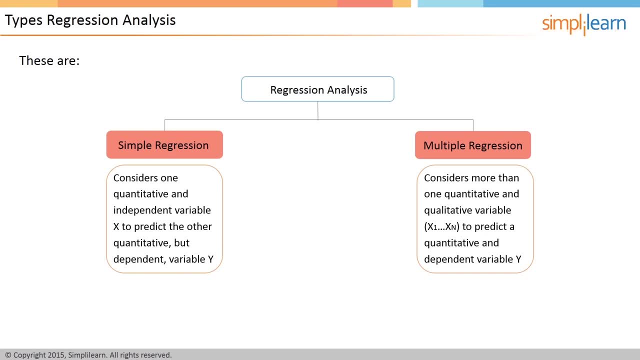 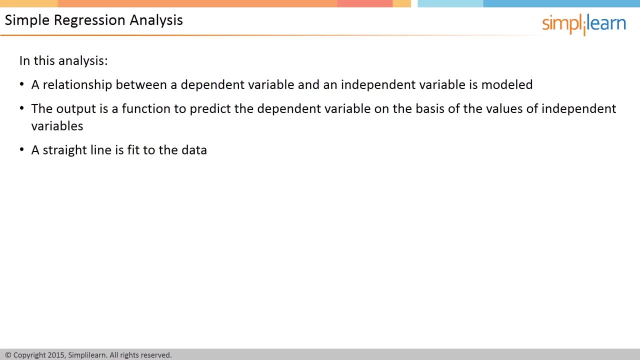 We'll look at the two types of analyses in more detail in the slides that follow. In simple linear regression You have the explanation of the explained variable y when plotted as a function of the explanatory variable x from a straight line. 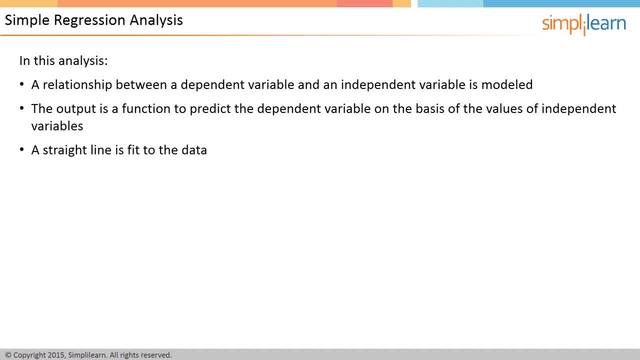 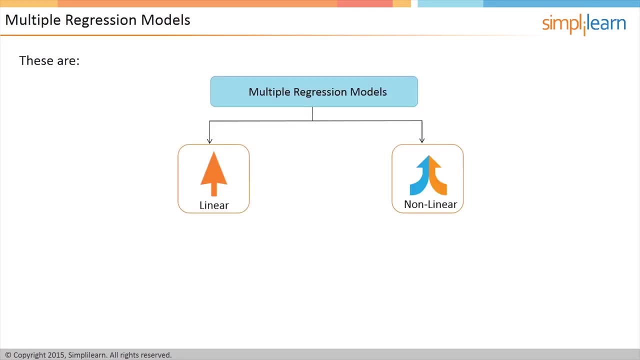 The best fitting line is called the regression line. The output of this model is a function to predict the dependent variable on the basis of the values of the independent variable. The dependent variable is continuous, and the independent variable can be continuous or discrete. Let's look at the different kinds of linear and nonlinear analyses. 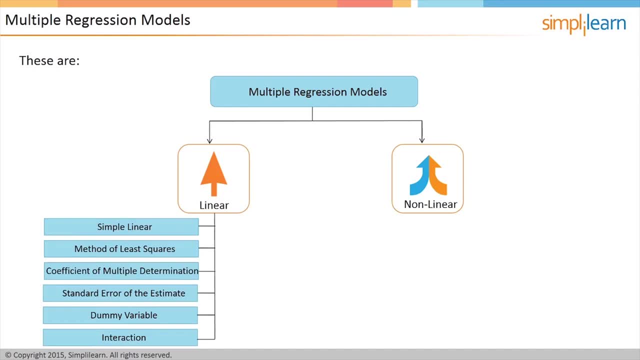 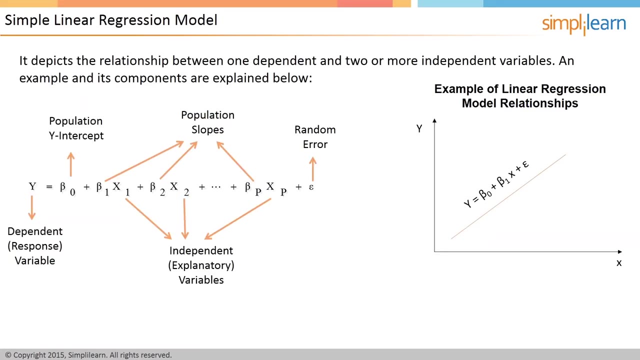 List of linear techniques are simple: least squares, coefficient of multiple determination, standard, error of the estimate, dummy variable and interaction. Similarly, there are many nonlinear techniques available, such as polynomial, logarithmic, square root, reciprocal and exponential, To understand this model. 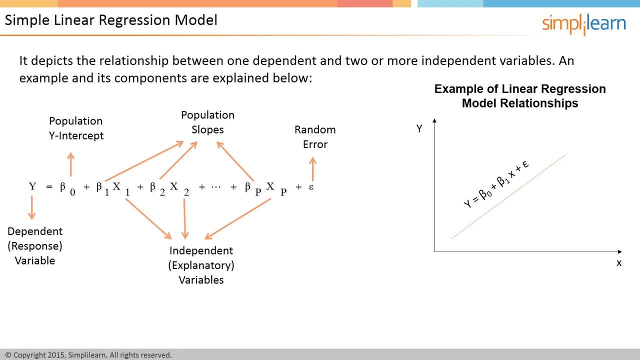 we'll first look at a few assumptions. The simple linear regression model depicts the relationship between one dependent and two or more independent variables. The assumptions which justify the use of this model are as follows: Linear and additive relationship between the dependent and independent variables. Multivariate normality. Little or no collinearity in the data. Little or 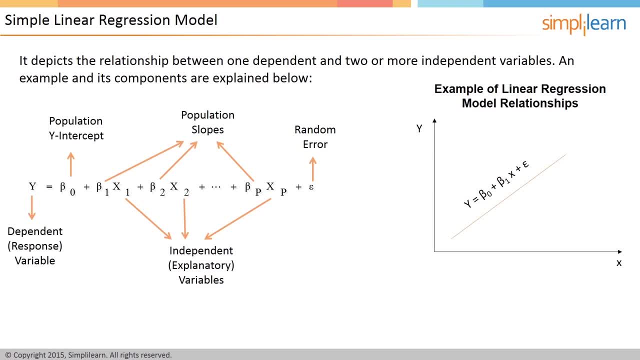 no autocorrelation in the data. Homosedasticity, that is, variance of errors, same across all values of x. The equation for this model is shown on the screen. A more descriptive graphical representation of simple linear regression is given on the screen. 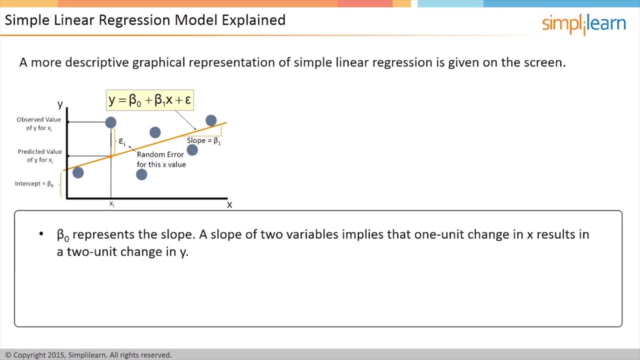 Beta naught represents the slope. A slope with two variables implies that one unit changes in x result in a two unit change in y Beta. one represents the estimated change in the average value of y as a result of one unit change in x. Epsilon represents the estimated average value of.